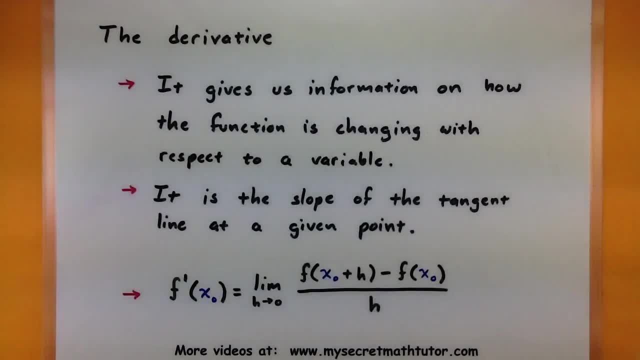 formula gives us that information, And then, near the very end, we'll look at, say, the information that tangent line gives us in places where the derivative does not exist. Okay, so watch for that near the end. All right, so let's see what we can do with this. 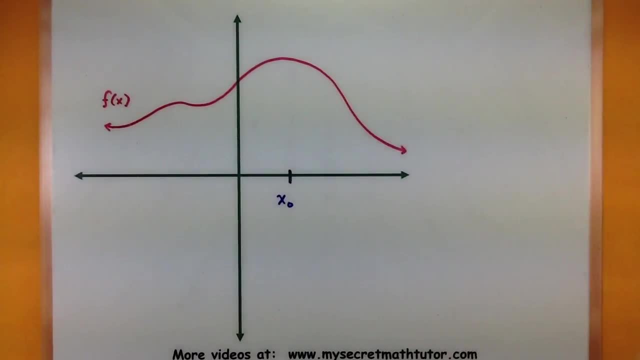 definition of a derivative. So imagine having some, you know, generic function, maybe something like this, and it could be increasing, decreasing, you know just doing all kinds of things. And what I'm really curious is: you know what is happening at this point? x sub zero. 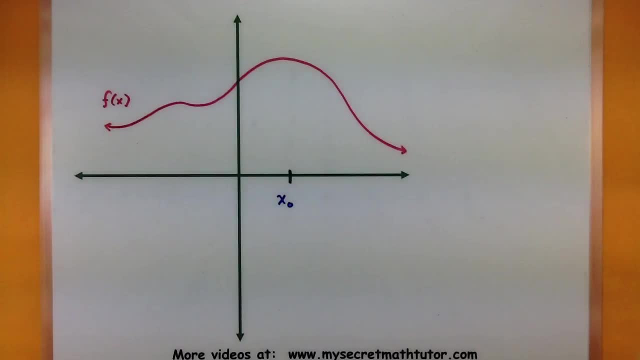 How is it changing? How is it changing at that specific point? Well, the only problem with finding that tangent line directly is: you know, if I want to figure out something like the slope, I need two points to do it. So what we do is we end up picking a second point a little bit further down and we do. 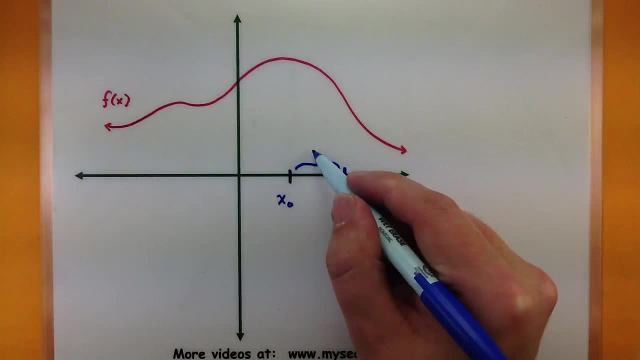 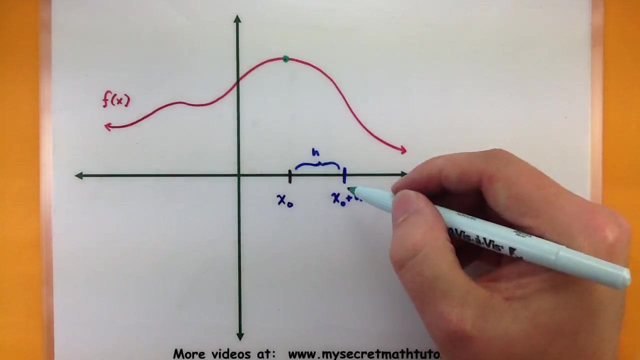 this at a distance of h away. Let's call the second point x sub zero plus h. If you want, you can mark the corresponding points on the actual graph. So there is a point right here. that's when we plug it into the function and we'll have. 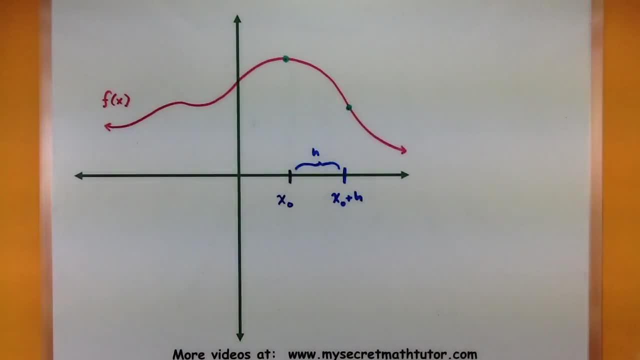 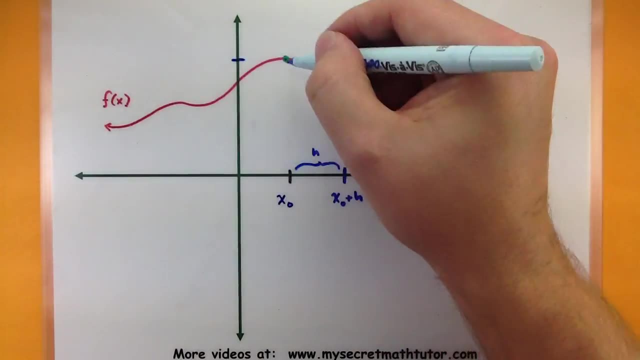 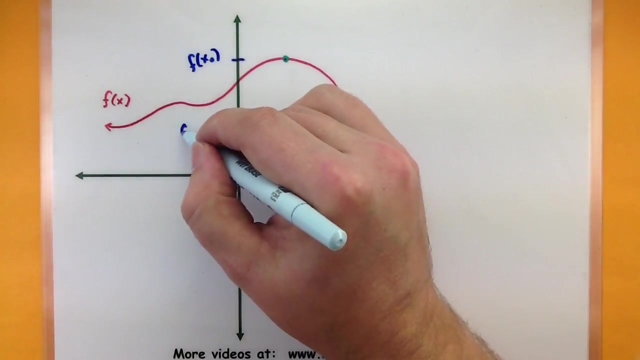 a point, say a little bit further down here, So let's mark out their y values. Okay, so this one way up here that's what happens when I put x sub zero in, and this one would be f of x sub zero plus h. 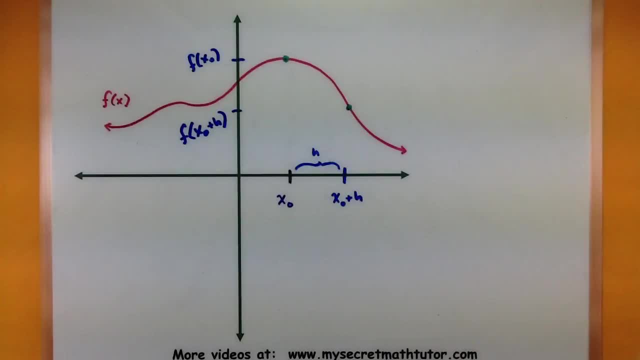 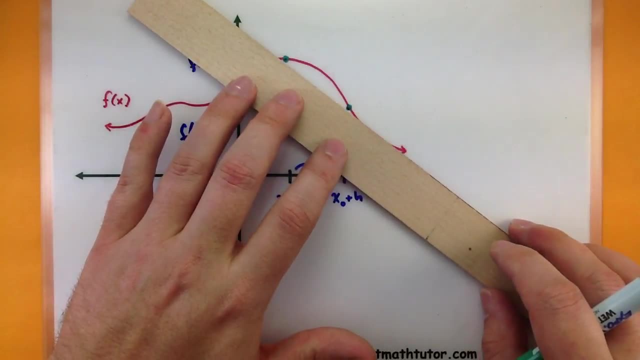 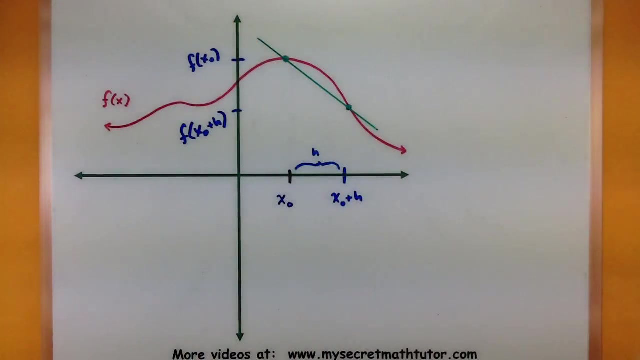 Okay. So in order to compute the secant line through these two points, we need to figure out the rise over run. So let me draw in our secant line and then we'll actually just write down the equation for the slope and eventually turn it into our formula for the derivative. 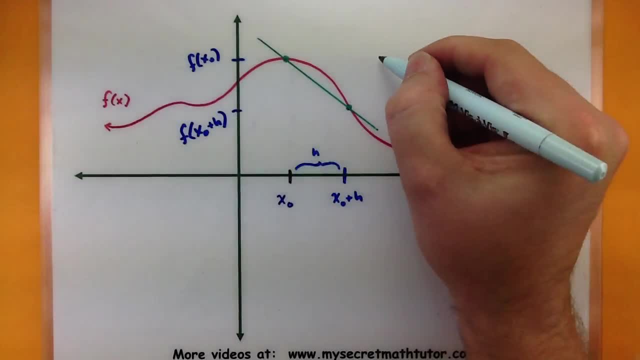 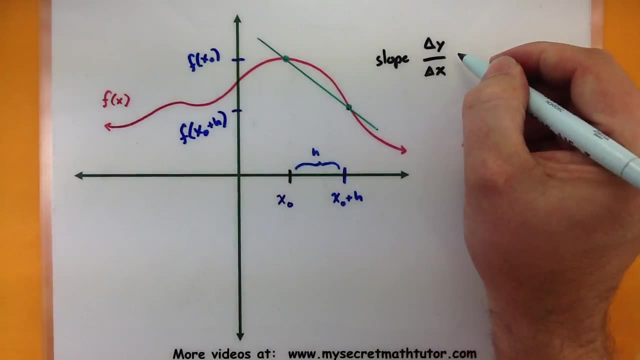 Okay, So to figure out slope, we're looking in the change in our y values all over the change in our x values. So to grab our change in our y values, we're going to take the slope and we're going to change in our y values. we would subtract the y values from each other. 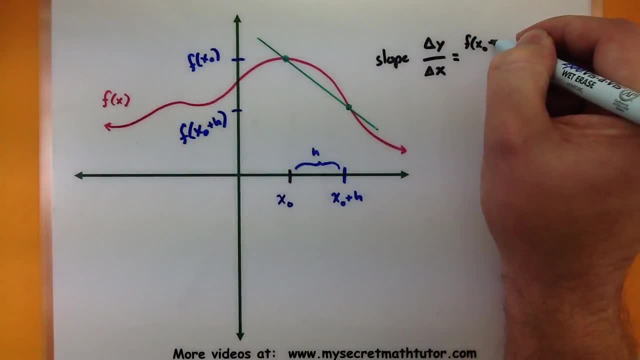 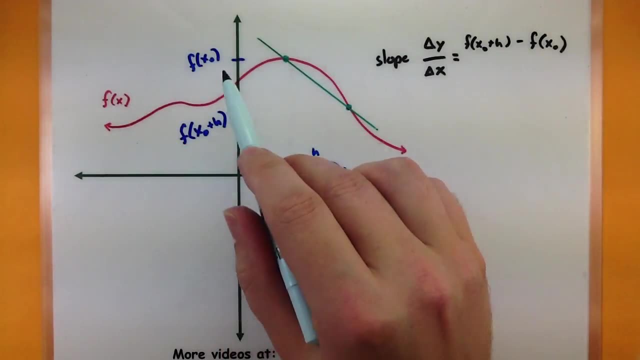 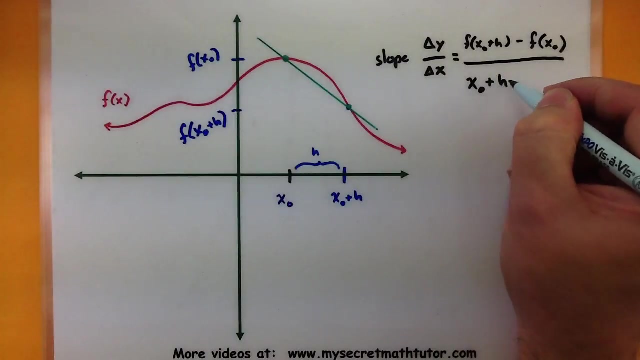 So imagine taking, say, the second point minus the first one, So f of x sub zero plus h minus the first one, And then we'll divide that by the x values, So this x value minus that x value. So this right here would give me the slope of the green line and it's kind of close. 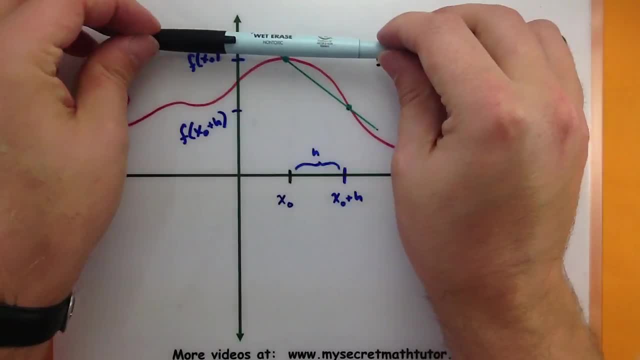 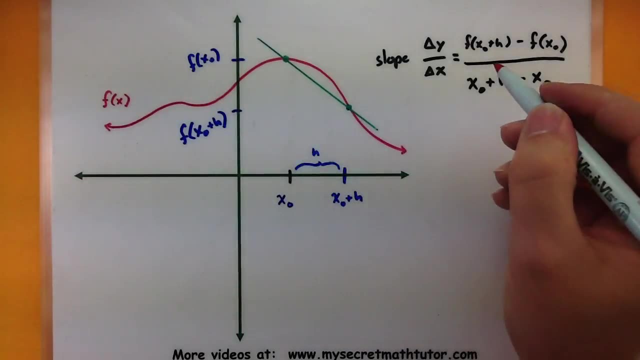 to the actual line I'm looking for. Remember that we're still actually interested in the tangent line up here, but you know what? The green line is pretty close. Well, we can do a little bit of simplifying with this guy, maybe cancel out some x sub. 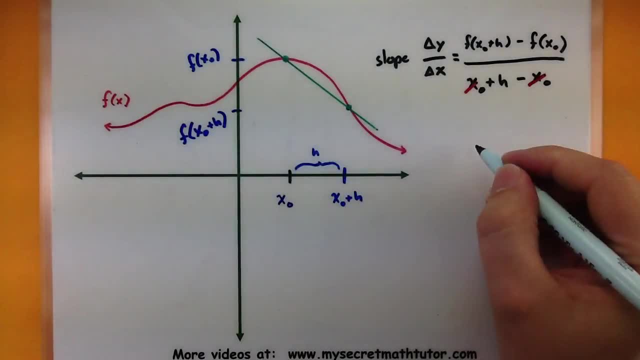 zeros, And you can see that we get this formula right here: f of x sub zero plus h minus f of x sub zero. Okay, Okay, Now, if I want to use this line to actually give me the slope of my tangent line, I need: 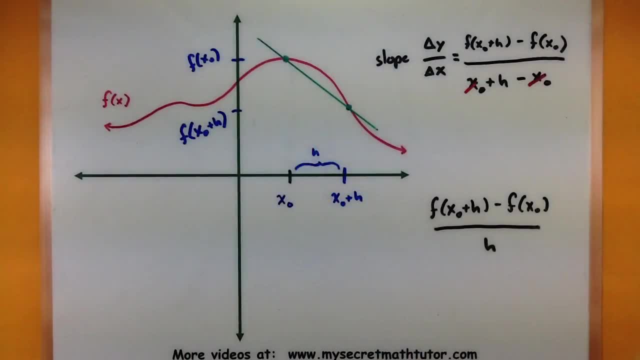 to get these points closer and closer and closer together until they're essentially just a single point. Well, the way we've made these two points is they are a distance of h away. So to really start squeezing them closer and closer together and get my tangent line, we 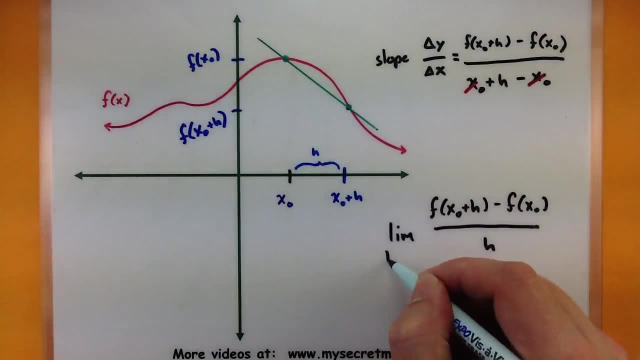 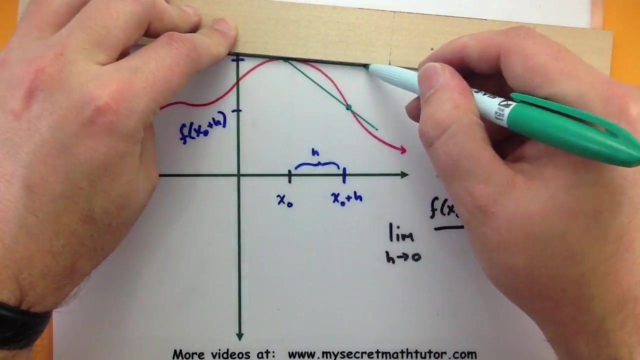 just add a small little piece to our formula so far. We say: let's see what happens when h goes to zero. All right, So imagining those points getting closer and closer and closer together, and that will build our tangent line. See, right about there. 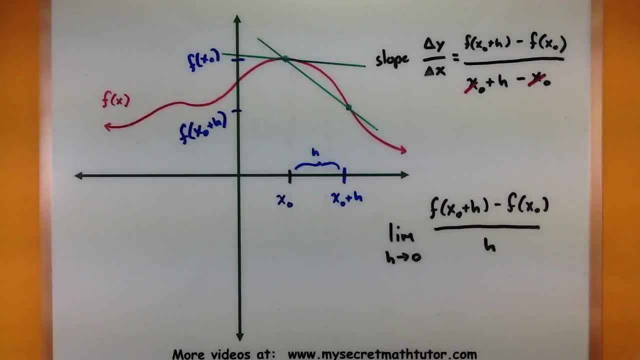 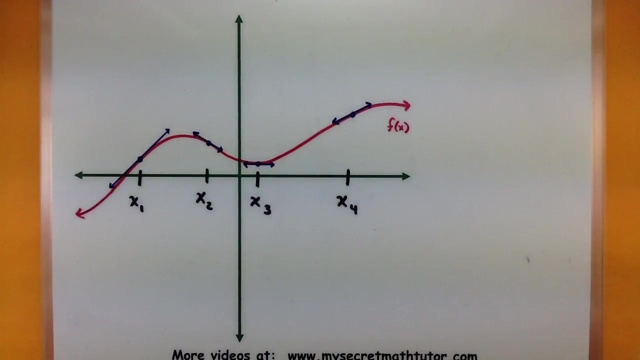 Well, that's what you know. exactly what we're trying to do with this formula is this: will tell us the slope of the tangent line at that specific point. We just have to compute a limit. So let's see How that tangent line really gives us information about our function. 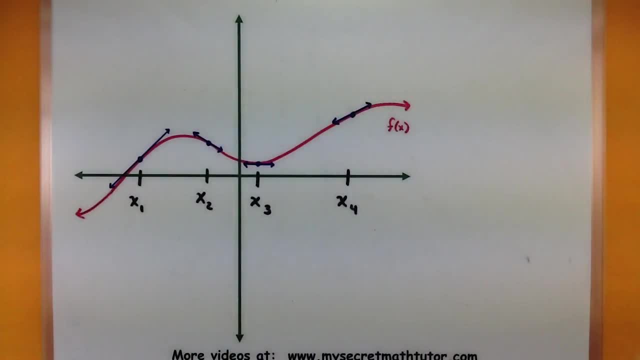 So here's another generic function. You can see that sometimes it's going up, Sometimes it's going down. I've marked out one, two, three, four specific spots on that function And in this first one you can visually see that tangent line is increasing, which corresponds. 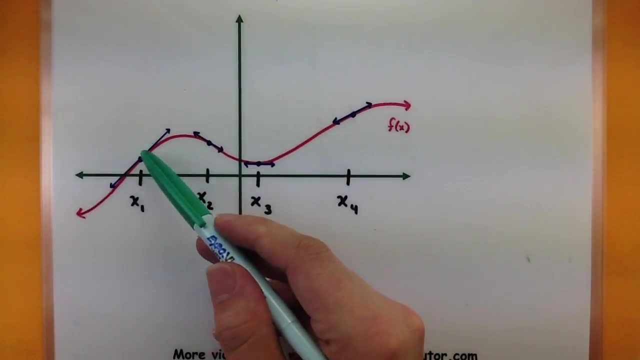 to what the function is doing. It's going up, And the steeper this line is, the more my function is actually increasing Here. So it's going down, So it would have a negative slope And sure enough, that corresponds to my function, which is decreasing. 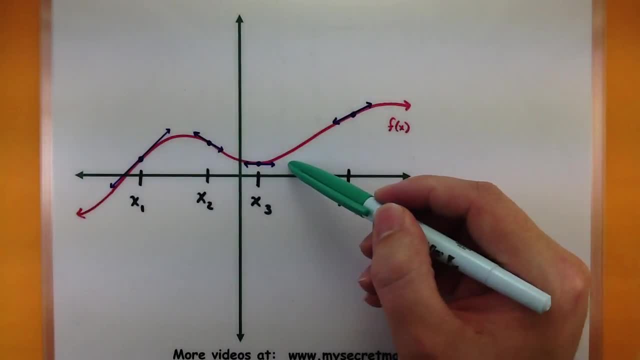 It's going down. Now, these tangent lines are also really good at finding places where your function really isn't going up or down. you know, staying the same value And notice how there the slope is actually zero. I got one more point just to demonstrate that actually the value of the slope does make 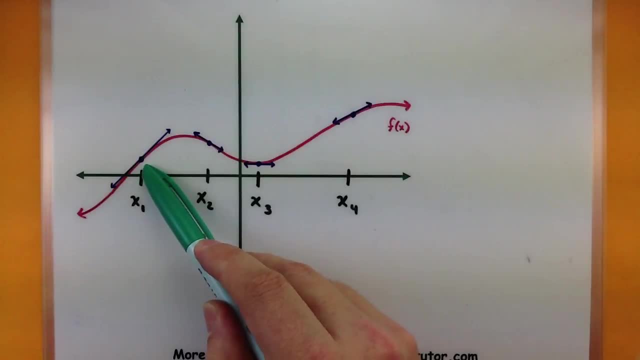 a difference on how much it increases. So our first point has a steeper slope. The second point has a deeper slope than this one, And sure enough, that's because the function is increasing more over here than it actually is over here. So, as you can see, the derivative gives us information about what our function is doing. 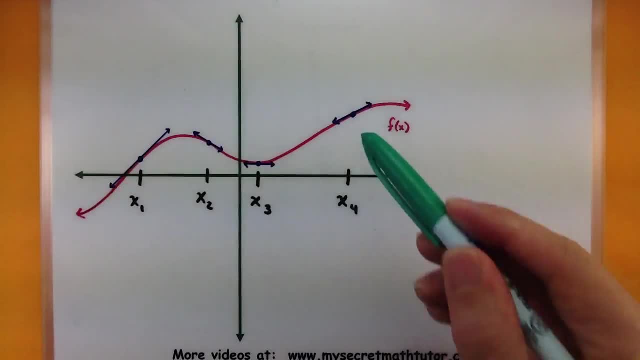 how much it is changing. And we're getting that information from the slope of the tangent line And to compute the slope of that tangent line, we look at the limit of the secant lines as they get really close to that point. Okay, so that's a lot of information about the derivative. 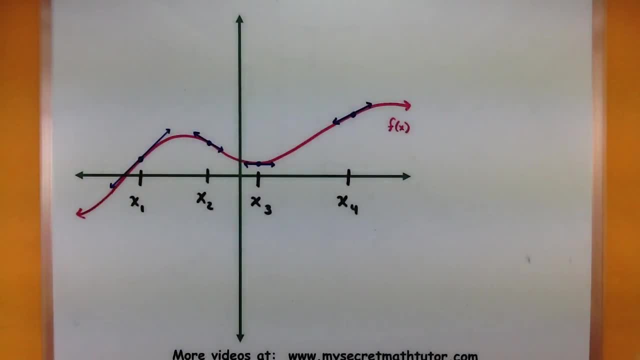 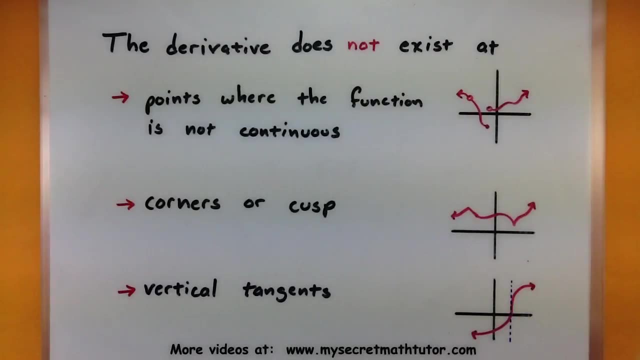 But unfortunately there are a few spots where the derivative does not exist. So let's look at the second point. Let's briefly look at some places where you know what you're not going to get a derivative, Since we're interested about specific points on the function and what's happening there. 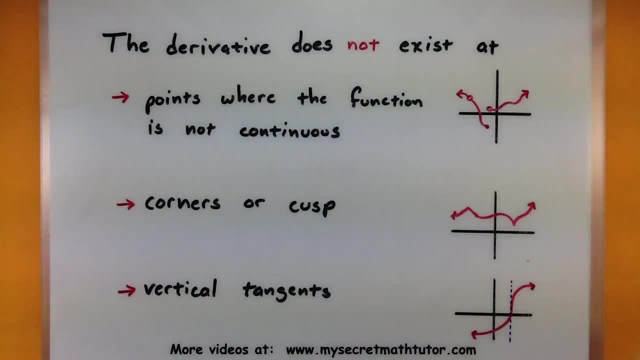 you can't have a derivative where the function is simply not there or where it's not continuous. So imagine your holes or your breaks or your gaps. if you have anything like that in your function, you can't build a tangent line there. 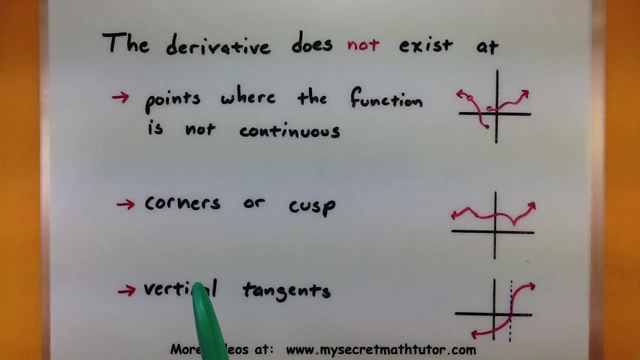 So derivative doesn't exist. Now, just because your function is continuous doesn't mean that your derivative doesn't exist. The derivative will always exist there either. In fact, the derivative does not exist at corners or cusps, So that'd be like this little corner or that little cusp down there. 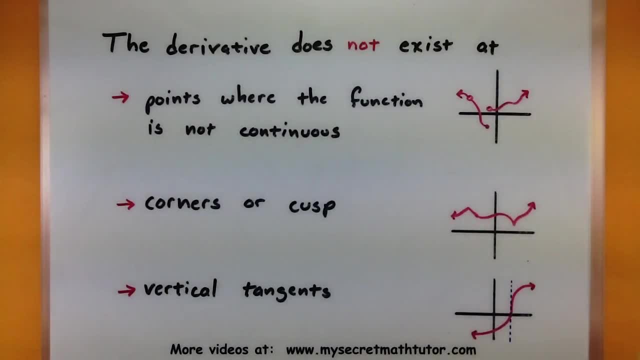 The derivative will not exist at those little points. Now, why not? What's going on? How come? Well, imagine what's happening, to say the tangent line, as you're getting really close to that point, but you're doing it on the right side.